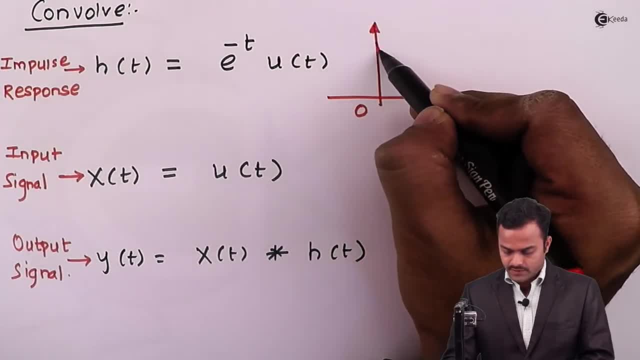 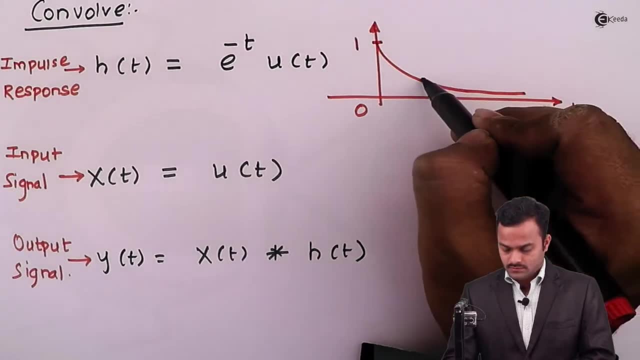 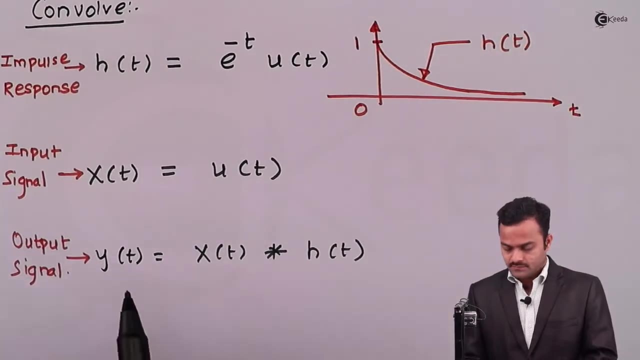 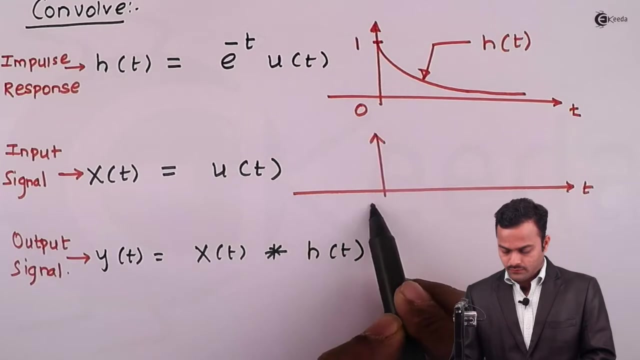 here it's a t axis and we will get a signal like this: So, at t equal to zero, it is having a value one. So this signal we obtained is h of t. x of t is a unit step, so it is quite easy. that means it will have the value one from zero to infinity, like this: 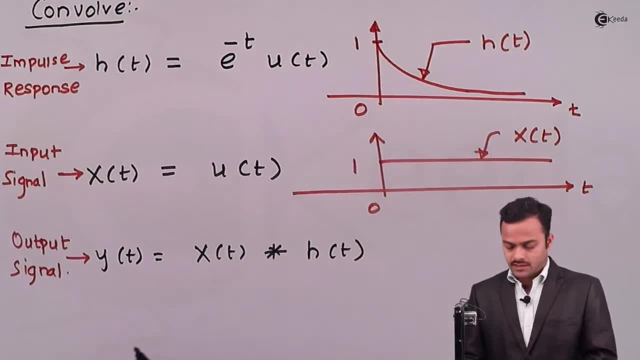 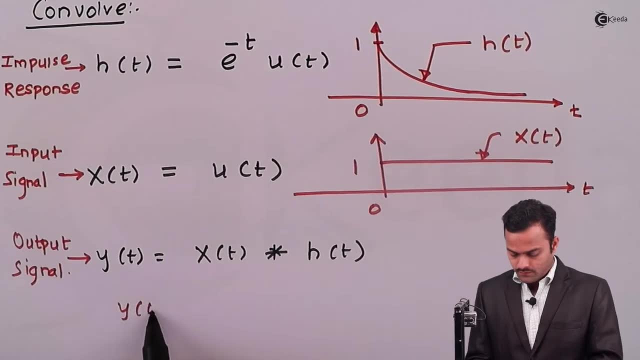 So these are the two signals given and we need to find out a convolution to get a y of t. So the formula that we are going to use is this: y of t is integral x of tau into h, of t minus tau into d. tau Limits will be from zero to t. In the end it is decided by. 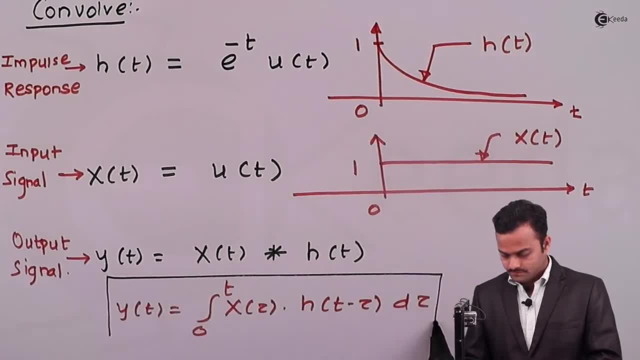 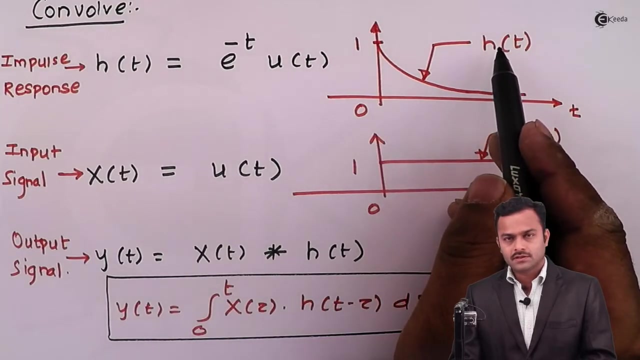 the area which is common between them. So let's solve it. The first step we are going to do over here is replacing t by tau, and at the same time I will do one more step, that is time reversal of this or this. So I will consider a time reversal of h of tau. So we will get a signal like this: 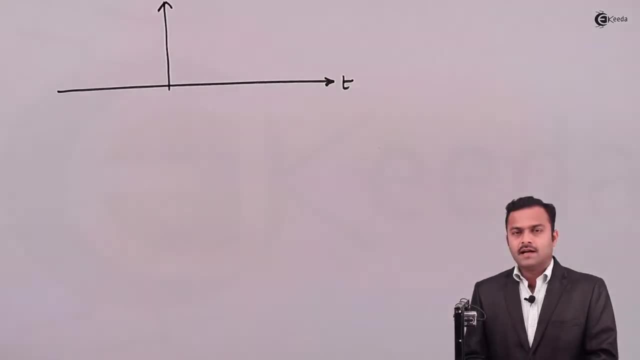 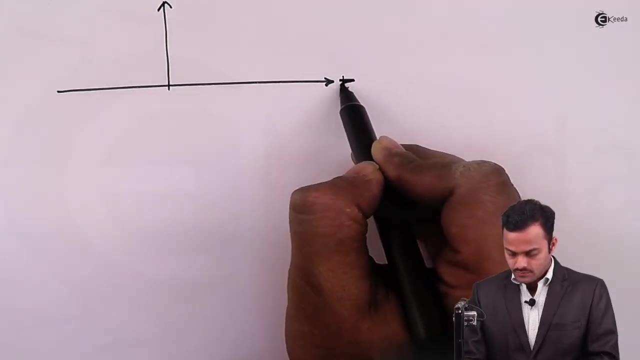 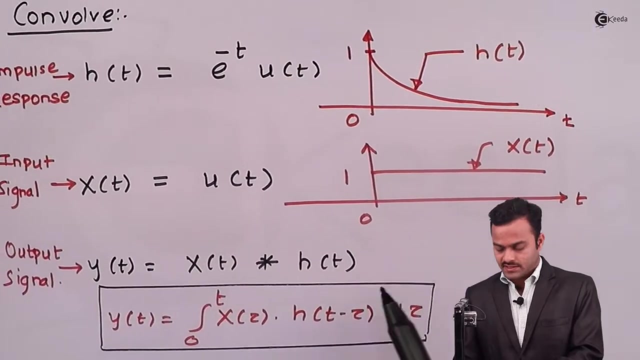 As we discussed earlier, we are going to consider this t axis as tau, so it will be like this: it's tau and then this tau here, x of tau. we are keeping as it is and we are just taking a time reversal of h of tau, So x of tau. as it is. so it will be like this: 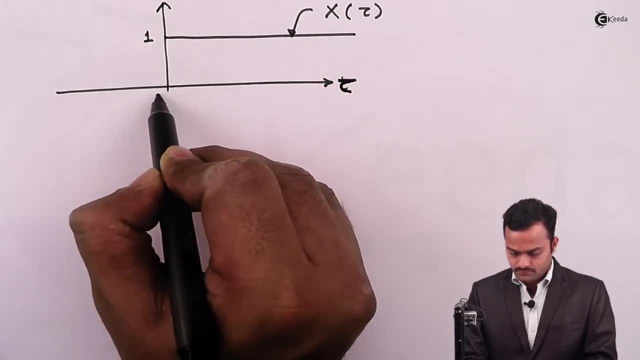 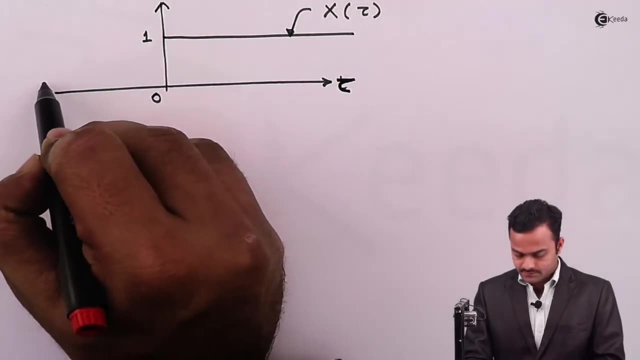 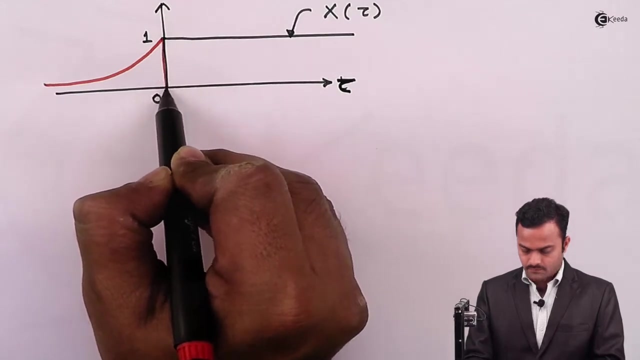 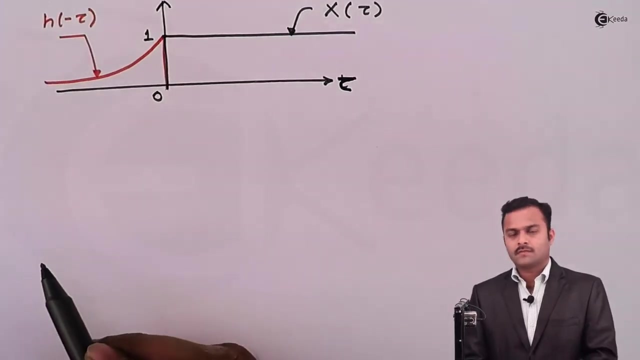 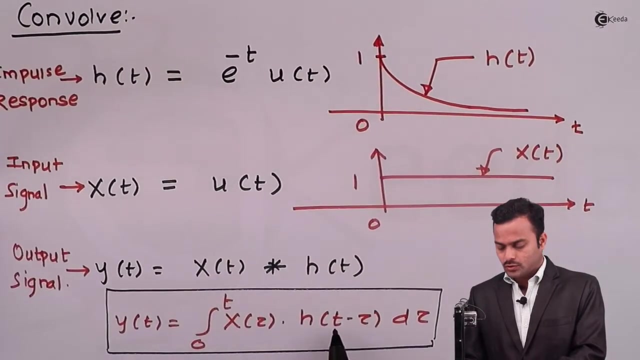 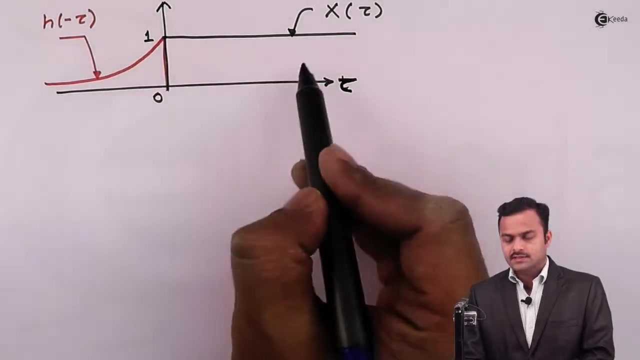 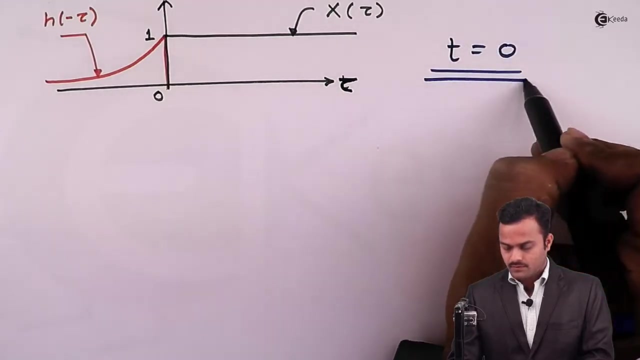 And h of minus tau. we will get like this Now: h of minus tau. if I compare with this, I will come to know: if I put t equal to zero in this, I will get h of minus tau. So in other words, I can consider this phenomena or this particular case where shift is zero, t equal. 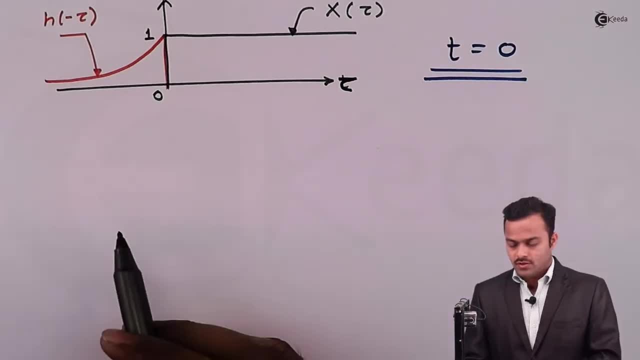 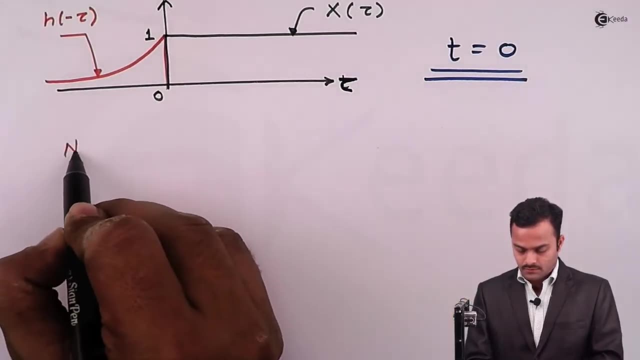 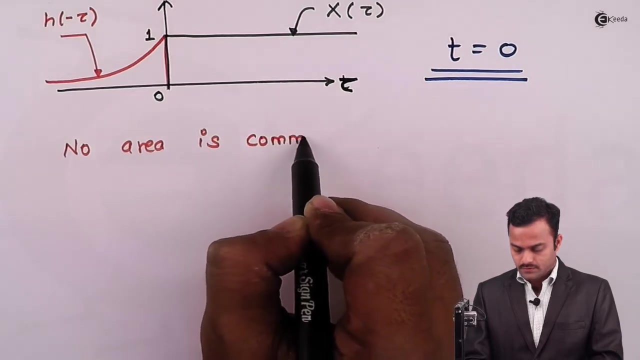 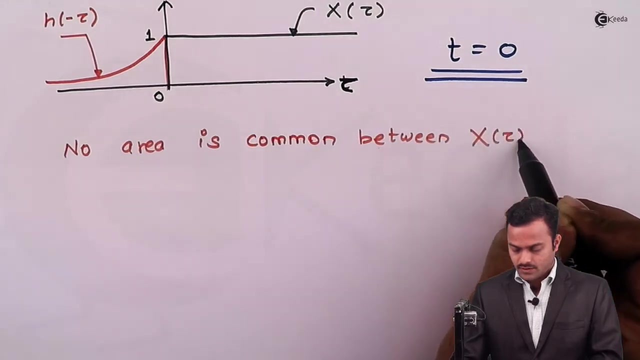 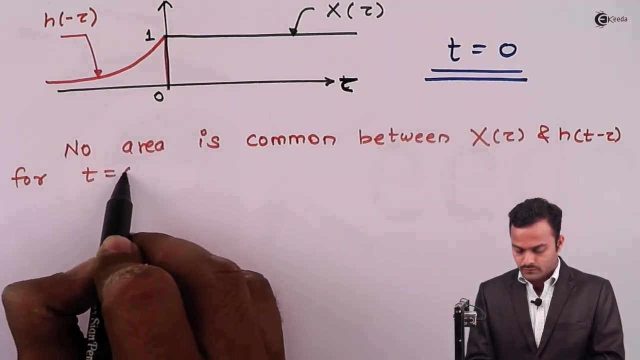 to zero. Why we are doing this? because we will be getting y of t at t equal to zero here itself, where we can say: no area. Now, h of minus tau is common between h of t minus tau and x of tau, So t equal to zero. 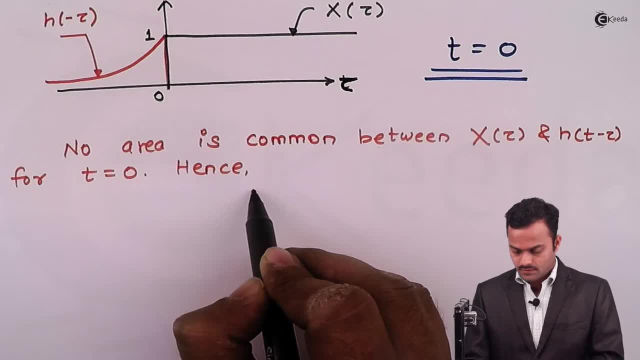 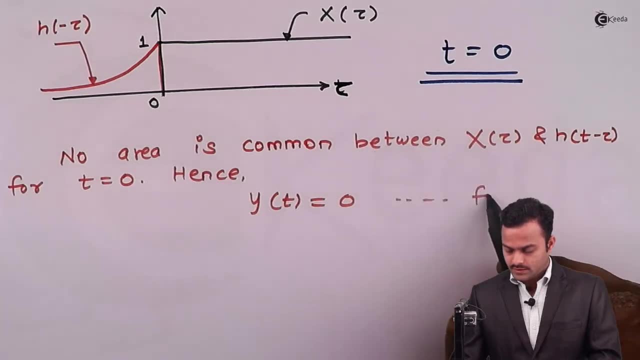 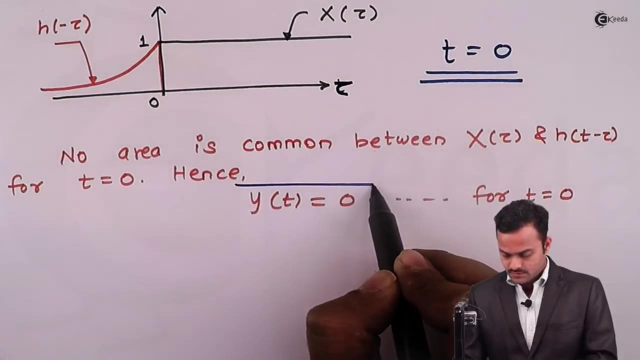 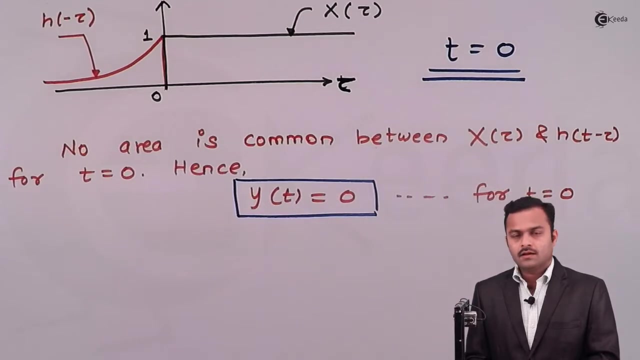 Hence I can say y of t equal to zero, straight away the condition apply. that is only applicable when t equal to 0, so we are getting a first output for 0, shifting like this. moreover, what I will do now I have reverse this, so I will. 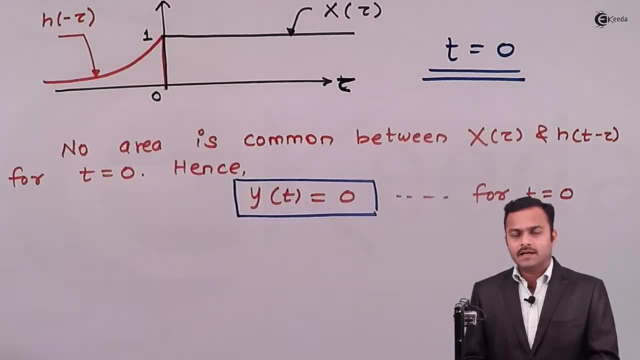 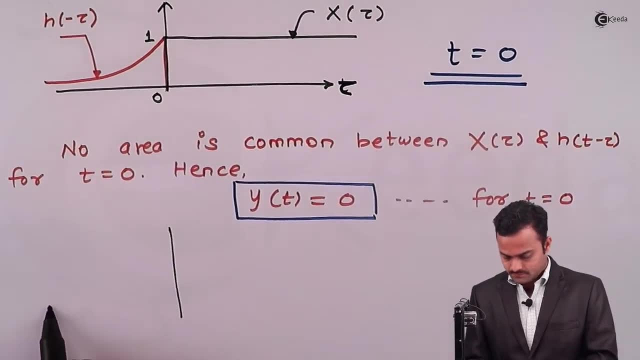 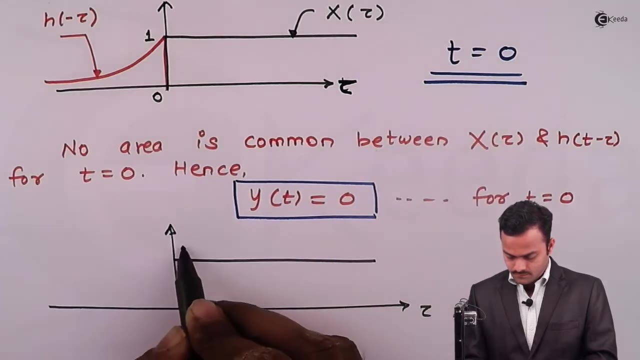 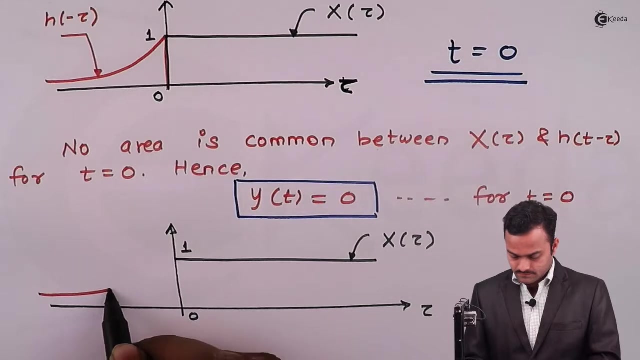 delay this sequence first, and I will delay it by any amount- t- so the resultant signals will look like this: this is x of tau and I am delaying this by t amount, so we will get a signal like this: and I am delaying this by t amount, so we will get a signal like this: 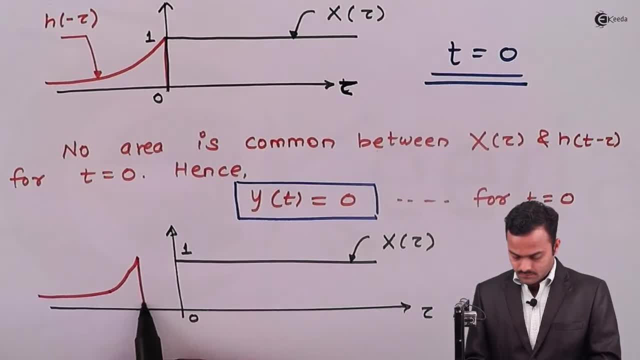 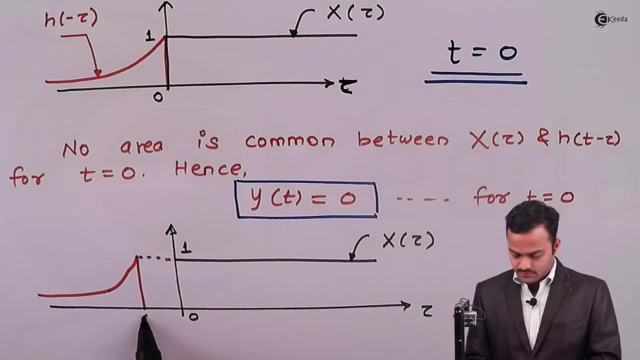 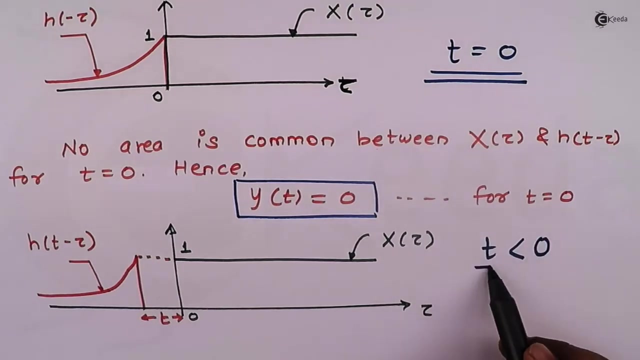 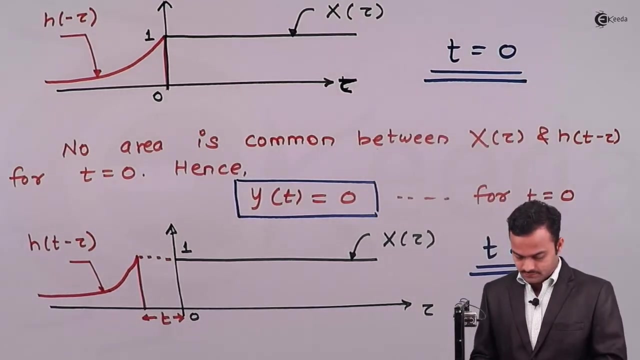 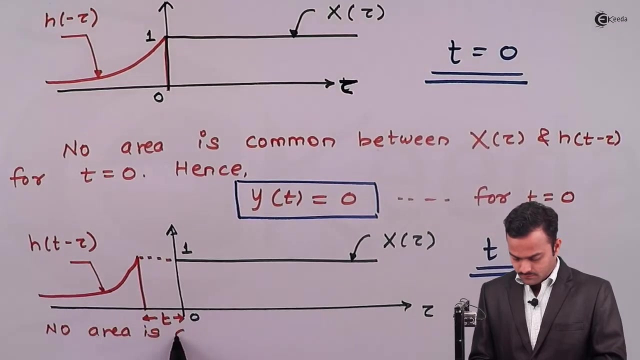 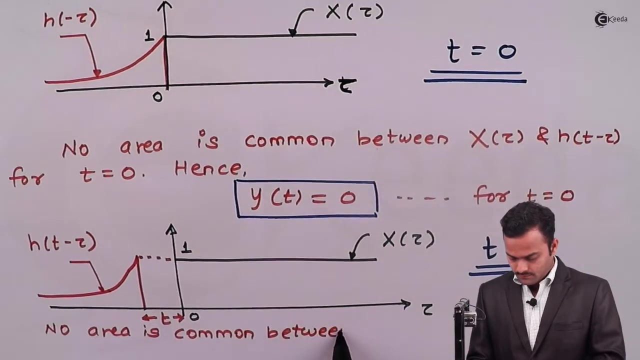 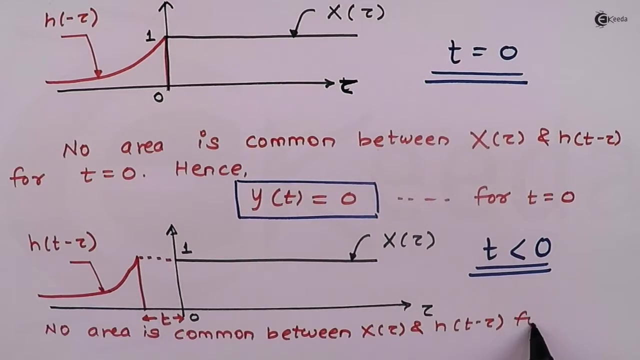 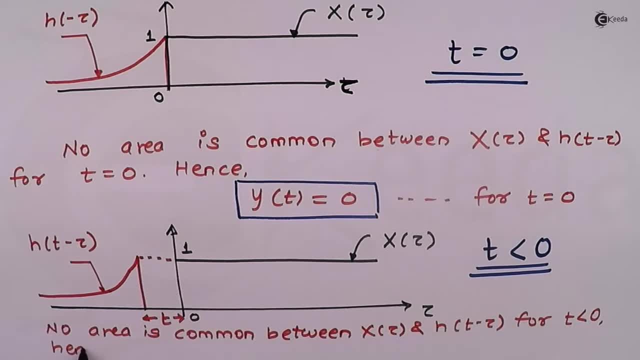 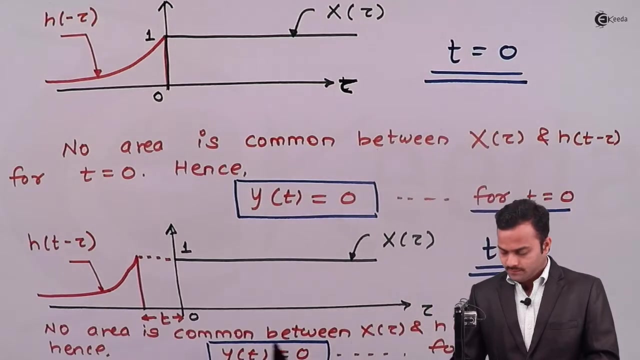 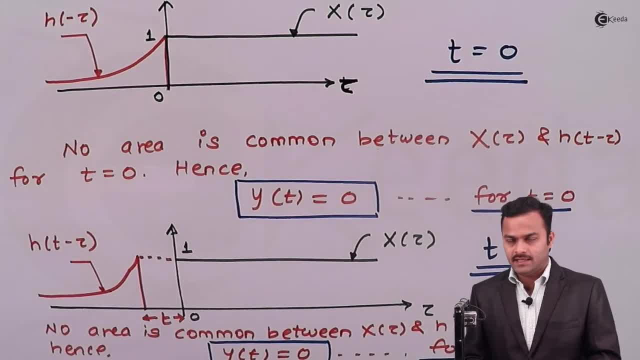 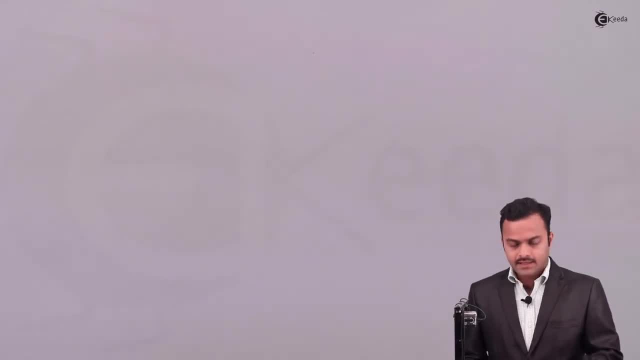 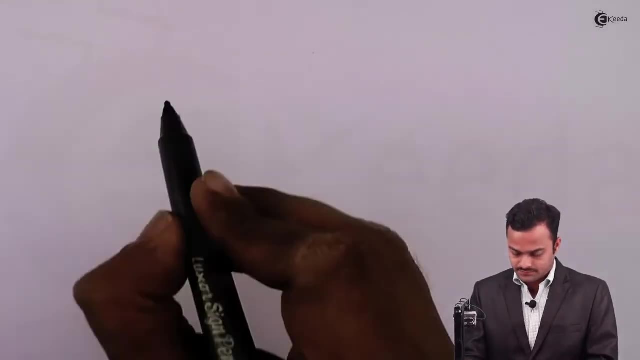 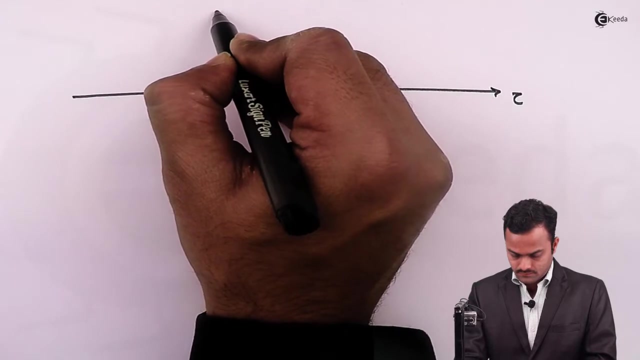 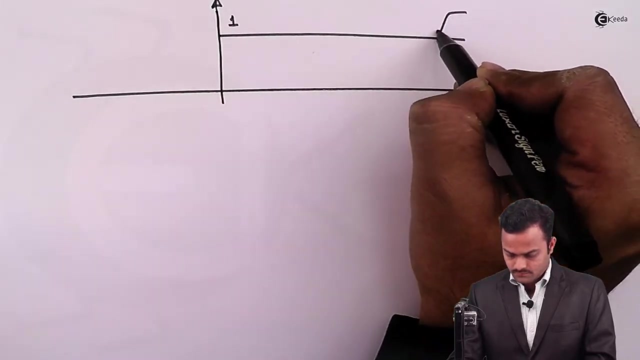 Now only case left is delaying this by any amount- t- So let's do it Now. what we are going to do, we are going to delay, repeat, we are going to advance Signal by t amount, so the resultant signal will look like this: Signal by t amount, so the resultant signal will look like this: 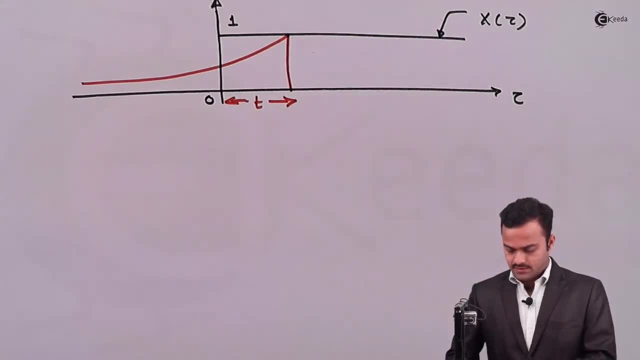 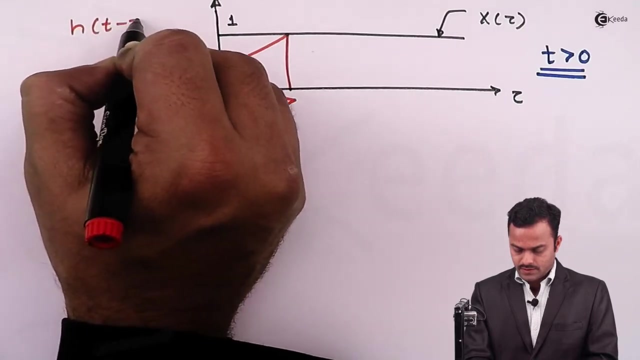 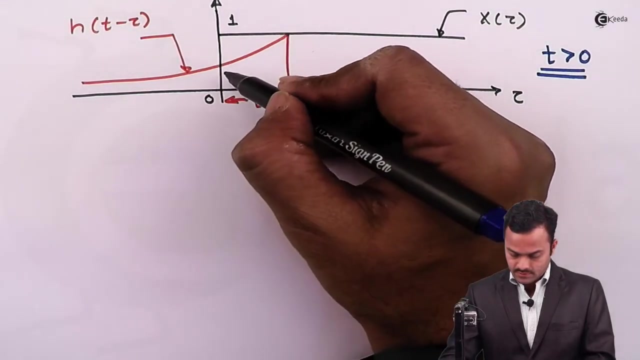 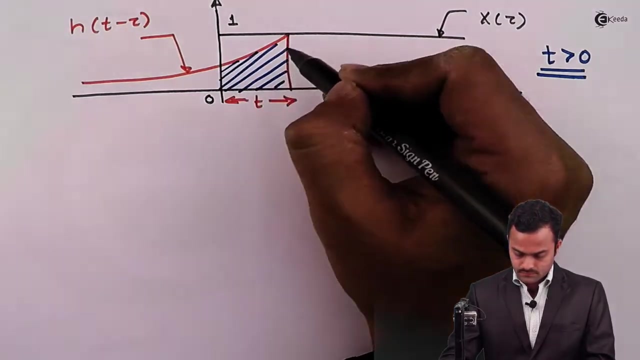 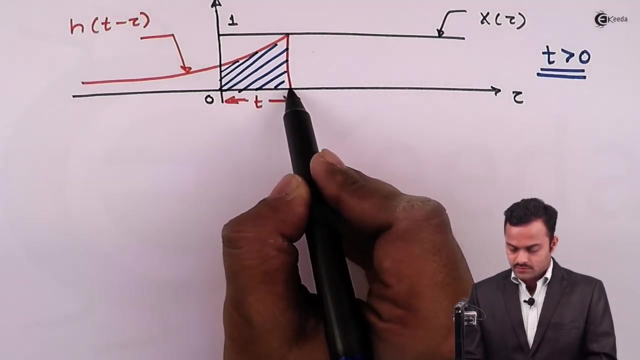 So this is shift, since we are advancing. advancing means what T is greater than zero And the signal that we obtain over here is H of t minus tau. So what we'll get over here, we'll get a area Common between these two signals like this. And, more importantly, what we are interested in knowing is what are the limits where the area is been formed? 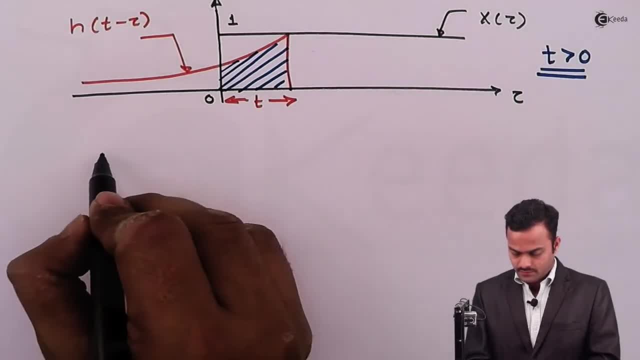 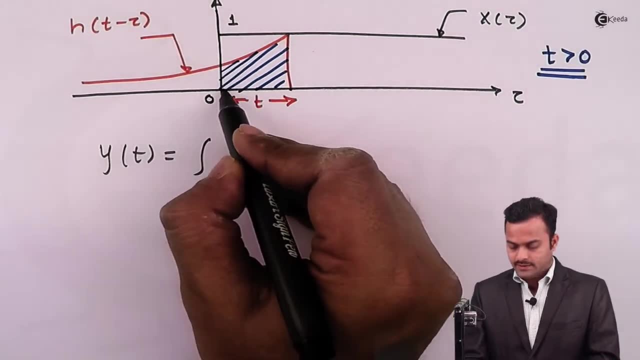 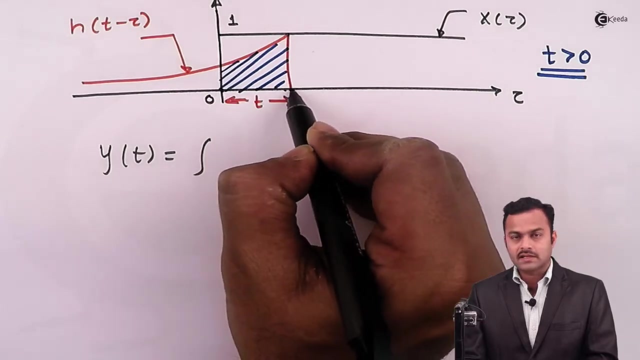 So since here some area is common, so we have y of t as integral, The integral limits will be decided by the limits of the area. So this is the area that we got. so here it is 0 and here it is t. so, but obvious, here it is 0 to t and 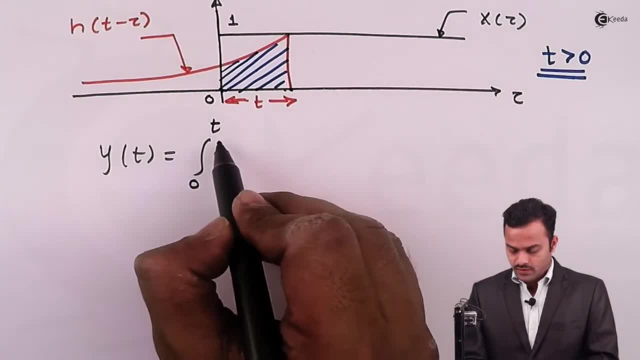 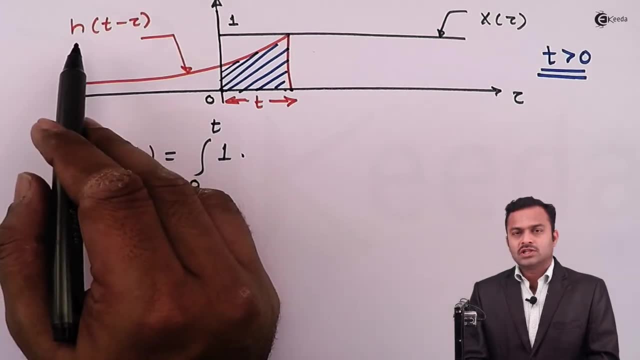 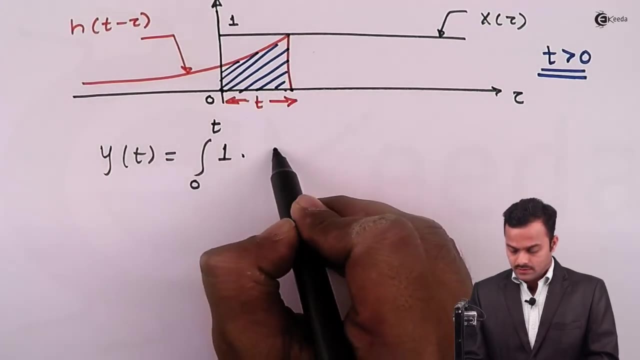 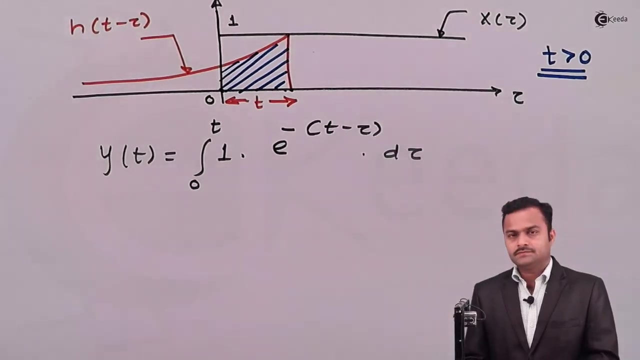 the value of x of tau is 1 only, but H of t, T minus tau, since H of tau is e raised to minus tau. Hence I will get H of t minus tau as e raised to minus t minus tau d tau. So I will get this expression and solving this integral will results in: 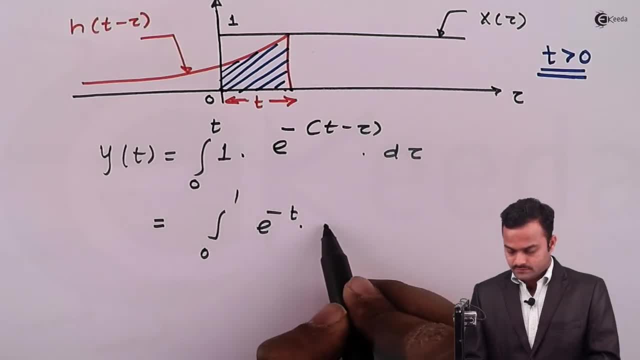 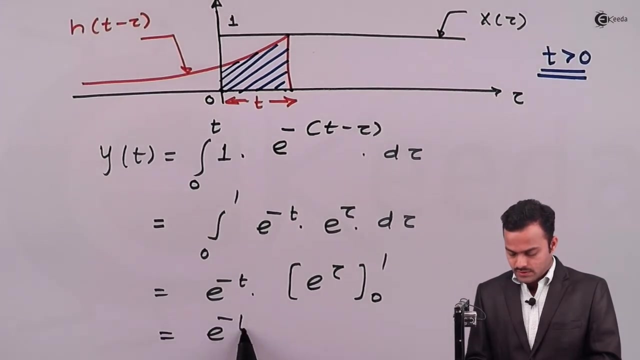 e raised to minus t multiplied by e raised to tau, d tau. So here is 2 minus t can be taken out and integral of e raised to tau is e raised to tau and The limits are 0 to 1. so if I apply the limits I will get e raised to minus t. 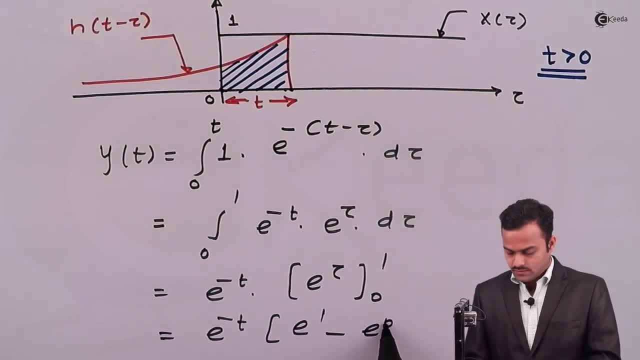 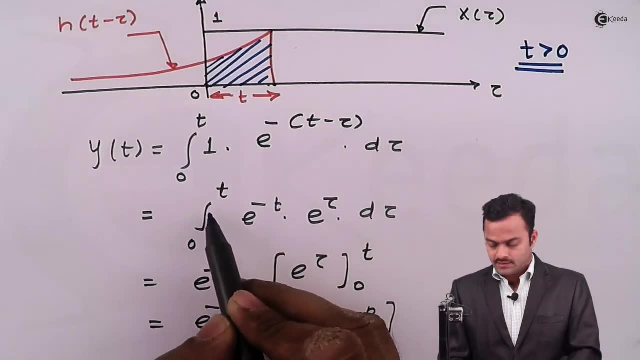 e raised to 1 minus e raised to 0. So solving this integral And simplifying, we will get e raised to minus t into e raised to tau limits 0 to t. And if you solve, since e raised to minus t is a constant, I can take it out of an integral. 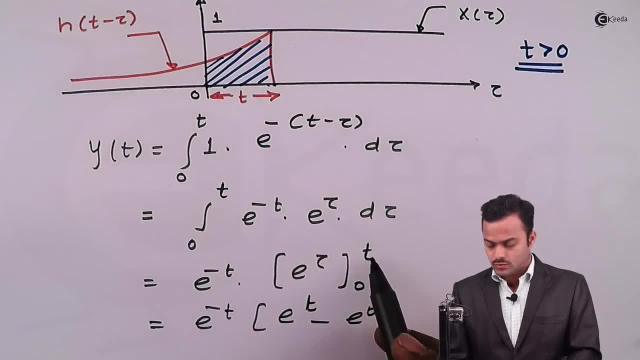 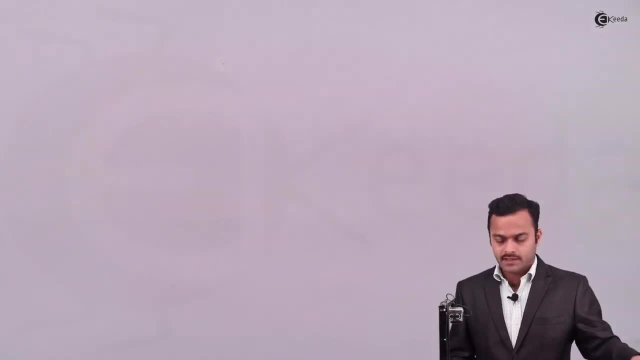 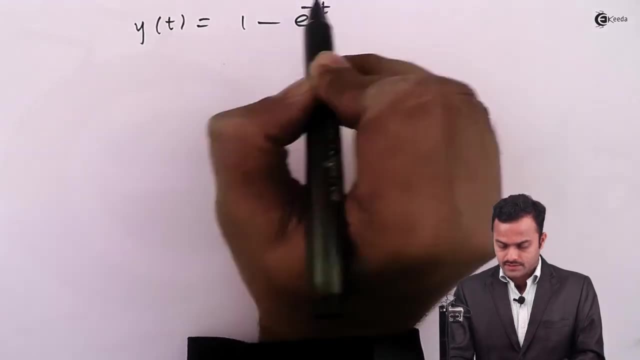 e raised to tau. integral is e raised to tau. limits are 0 to t. so if I apply the limits, we will get this expression, which further reduce, and we will get y of t as 1 minus e raised to minus t, and This is for t greater than 0. 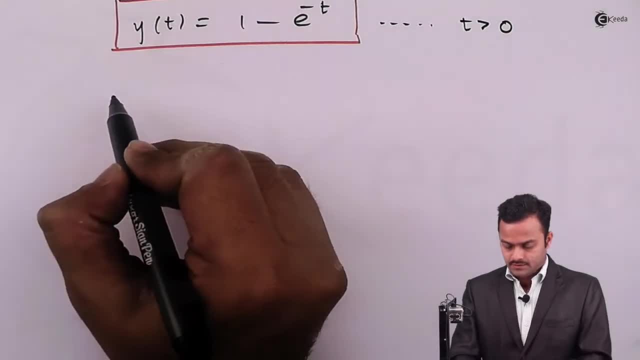 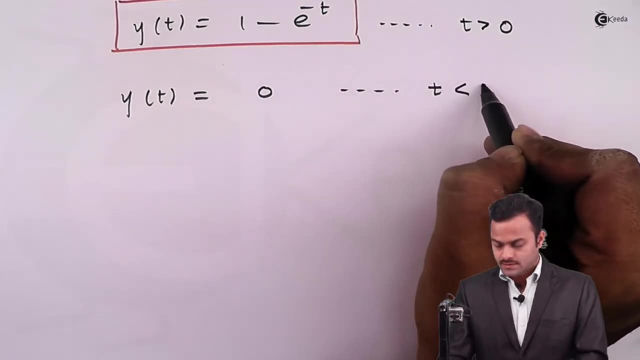 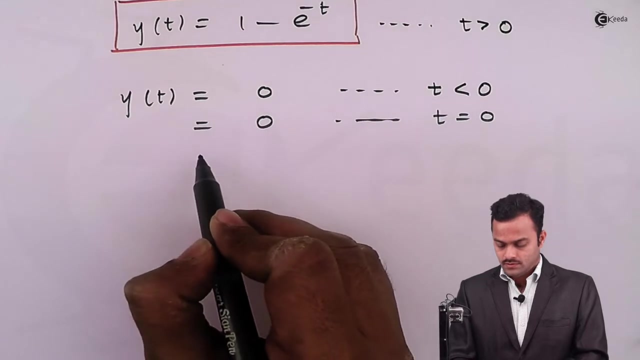 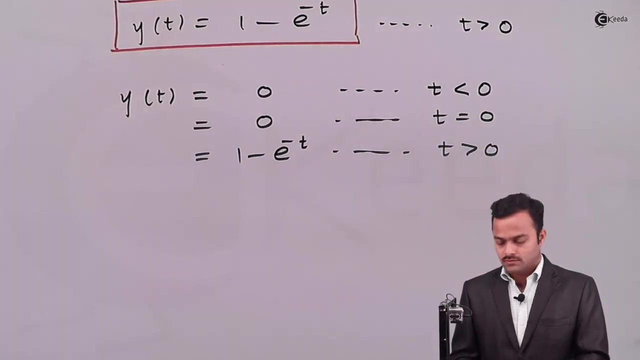 So now I'm having y of t, Which is equal to 0 for t less than 0. This is equal to 0 for t equal to 0, and y of t is 1 minus e raised to minus t For t greater than 0. so using this information we can plot y of t. 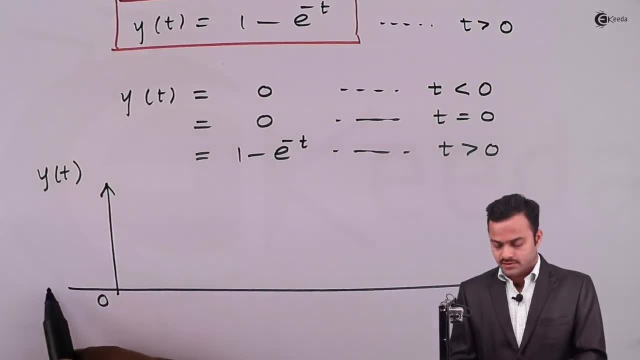 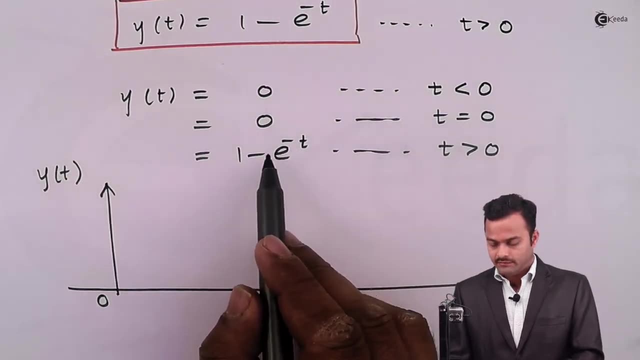 So it's quite simple: for t is less than 0, Then 0. for t equal to 0 is also 0. if I put t is minus infinity, I will get the ال. i will get the value as 1 to get repeat. if i put t as infinity, i will get e raise to minus.